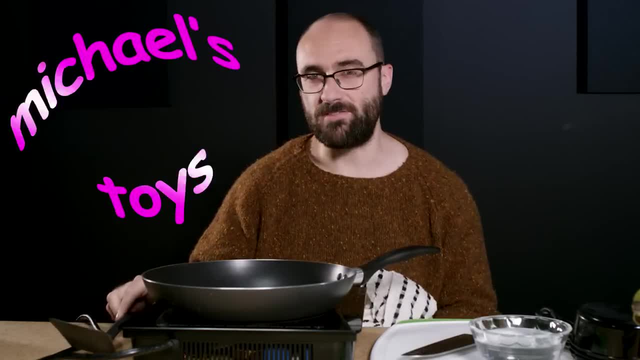 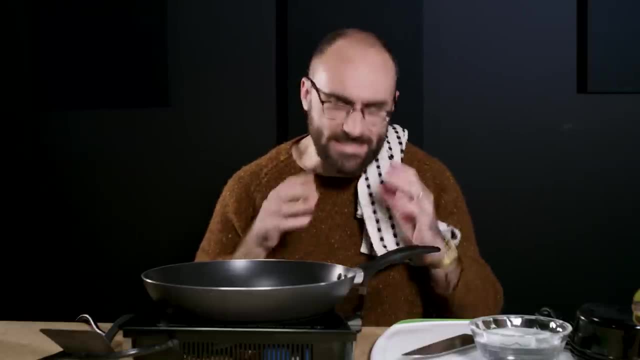 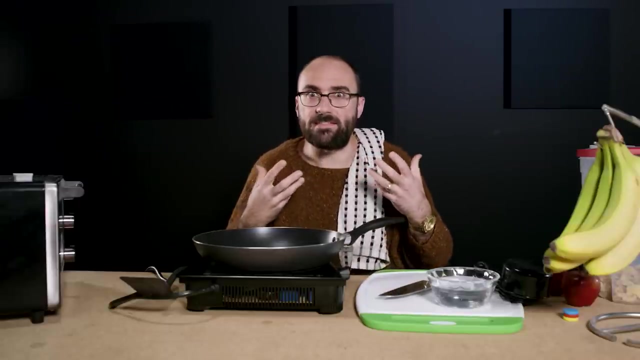 Oh, hello. Welcome to Michael's Toys, the first and only show on YouTube made by, of and for teenagers who like to cook. I'm your host, Michael Stevens, and today we are going to be talking about magnets, Specifically the strongest magnetic field my body has ever been inside. 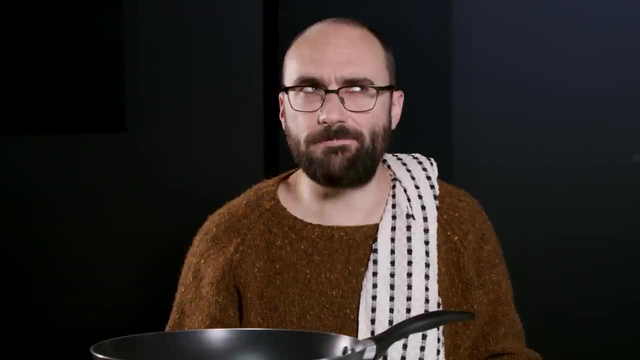 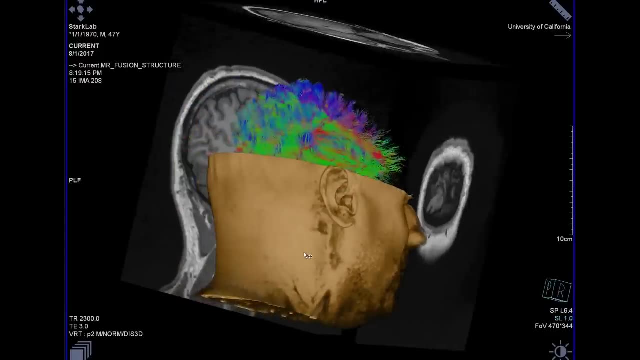 The 3 Tesla MRI at UC Irvine, Which I guess kind of makes this an episode of UC Irvine's Toys because they own the MRI. I don't. Anywho, I had a lot of MRI scans done of my brain for Mind Field Season 2, and I learned a lot about them and they are just beautiful and wonderful. 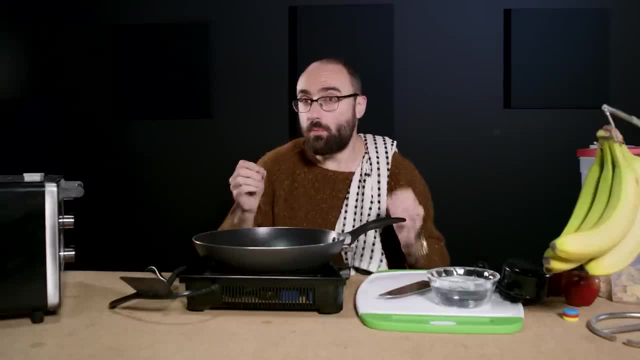 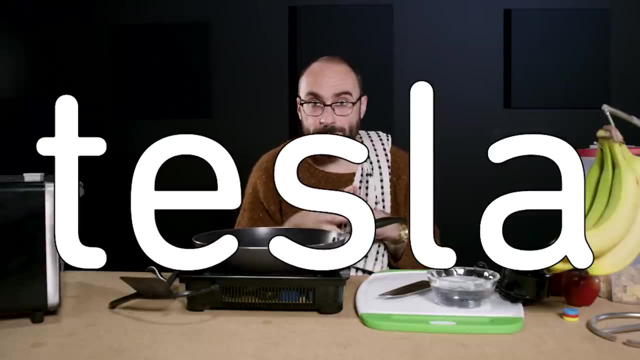 Here's a question: How strong are different magnets? Well, one way of measuring a magnet's magnetic field strength, really its magnetic flux density, is the Tesla. Alright, now to put a Tesla into perspective, our planet is a big magnet really. 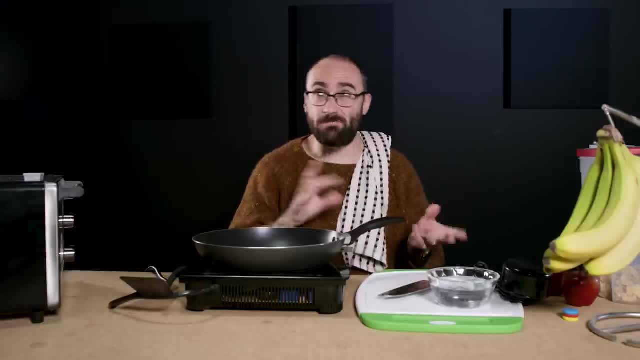 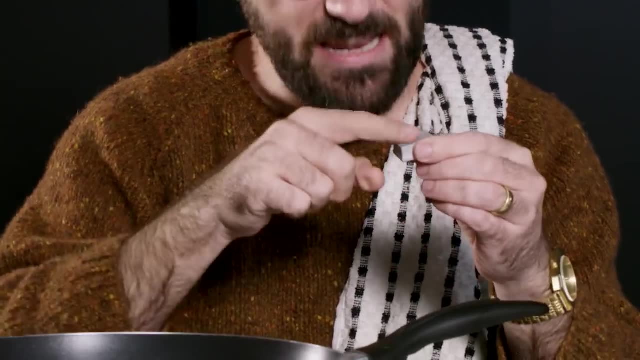 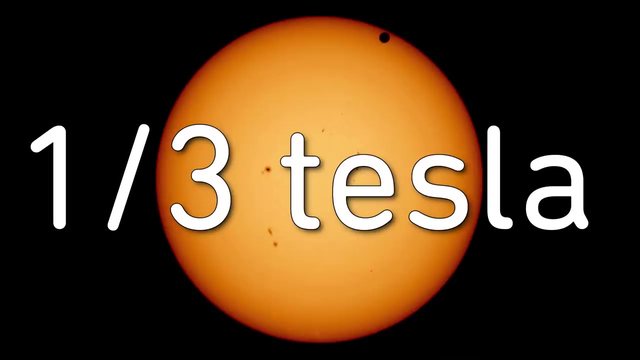 It's not a really strong magnet, though Its magnetic field strength is just about maybe 31 micro Teslas. In comparison, an everyday ordinary refrigerator magnet has a magnetic flux density of about maybe like 5 milliteslas. A typical sunspot can have a magnetic flux density of around a third of a Tesla. but the surface of a neodymium rare-earth magnet can have a magnetic flux density around 1.25 Tesla. The MRI machine I got in many, many times for Mind Field Season 2 was a 3 Tesla machine, Which means you can do some pretty weird things with it. 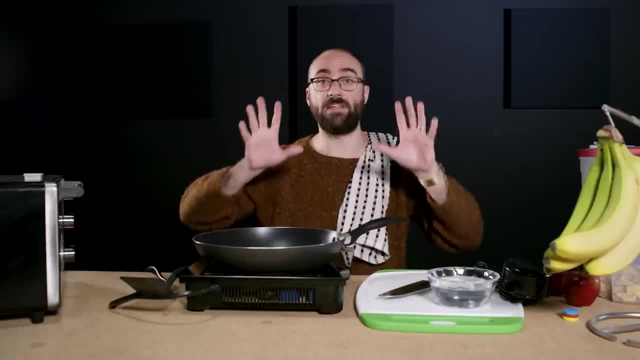 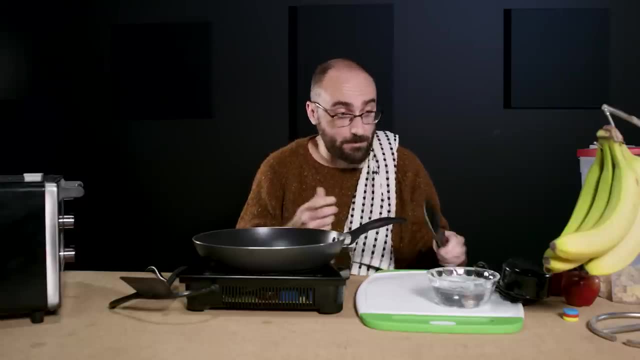 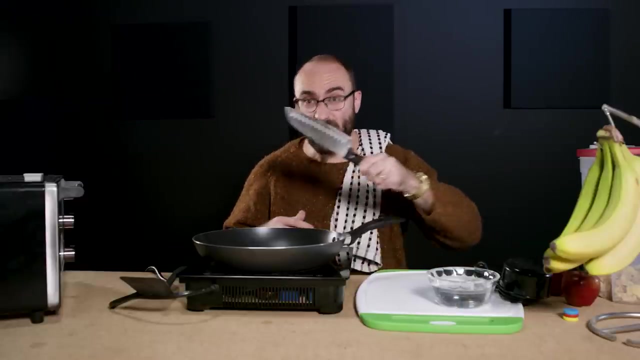 You have to be very, very careful. No ferromagnetic metals are allowed into the room it is in or even near it in the room outside, because it attracts ferromagnetic materials so quickly that they could be pulled from your hand, race through the air at an ever-accelerating rate until they strike the machine at like super lethal and at least very dangerous speeds. 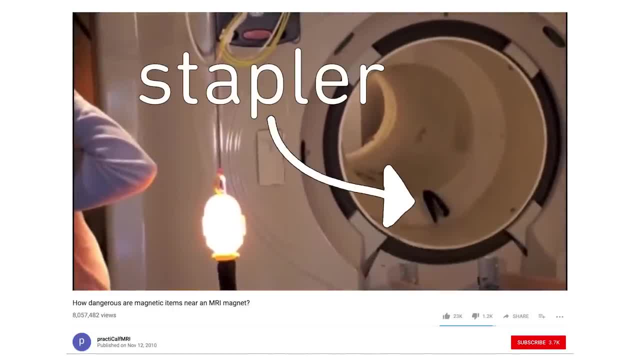 There are videos on YouTube where people show off just how dangerous the magnetic power of an MRI machine is. There are videos on YouTube where people show off just how dangerous the magnetic power of an MRI machine is. There are videos on YouTube where people show off just how dangerous the magnetic power of an MRI machine is. 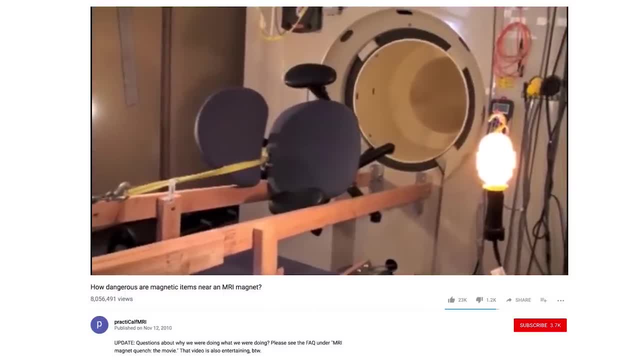 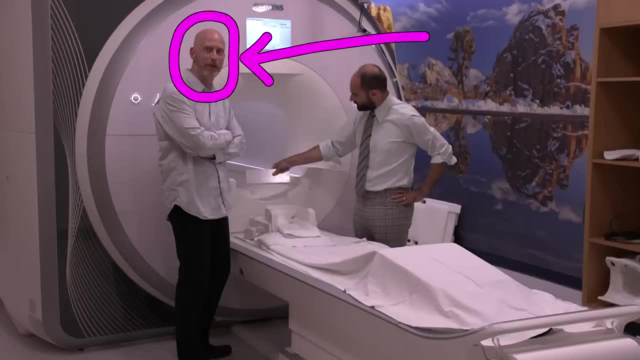 an MRI. an MRI can be. an MRI can be can lift chairs off the ground. But what about metals that aren't attracted to magnets? Well, they exhibit some very strange behaviors, and Craig Stark at UC Irvine was kind enough to allow me to bring in a giant block of Aluminum. 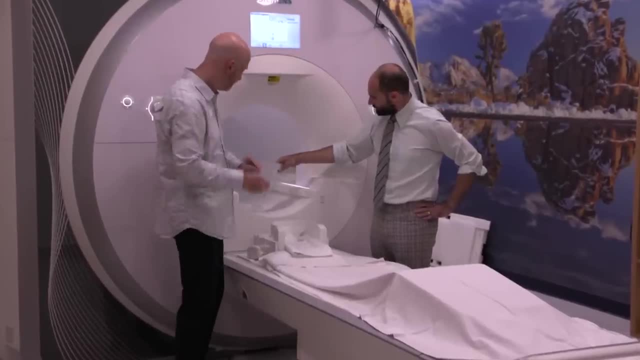 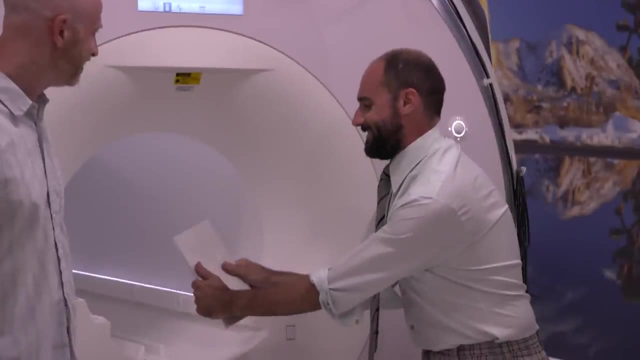 Now I'm gonna have to just talk over this clip because we obviously couldn't bring cameras or microphones to the room to pick up our voices. We had to set the camera far away and then zoom in to myself. Pause, Let's just take a brief moment to appreciate. 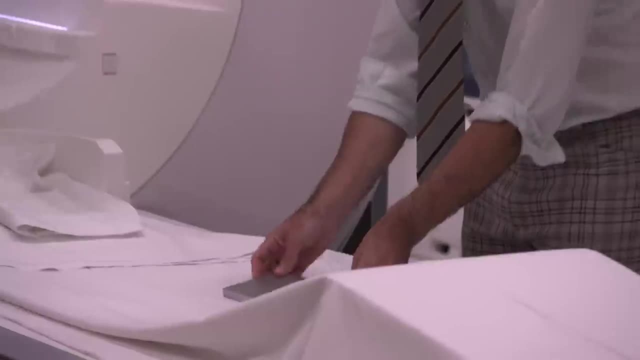 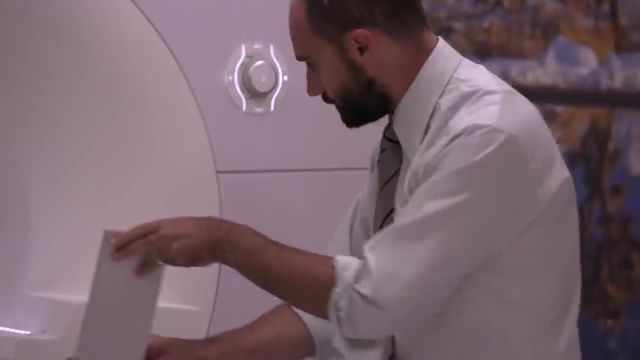 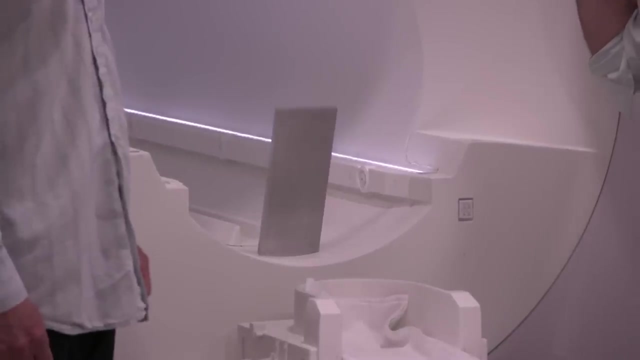 tan line on my face caused by my glasses. But here's an aluminum block and I'm going to set it up on its side and then let it fall. Ok, pretty easy. That's a great demonstration of gravity. but watch what happens when I set the aluminum block near the inside of the MRI and let it go. 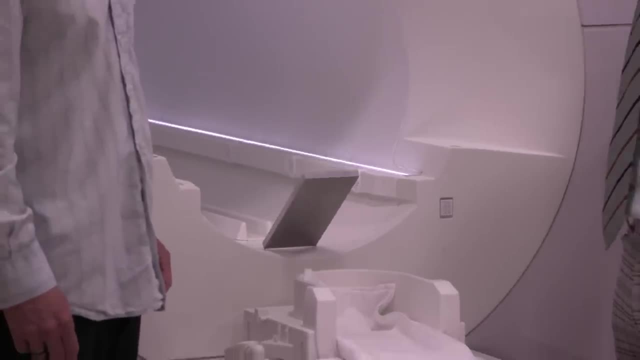 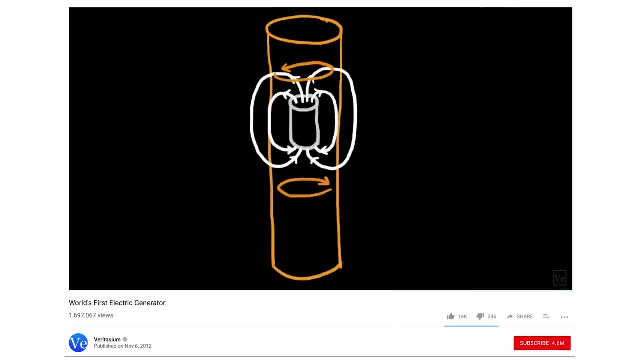 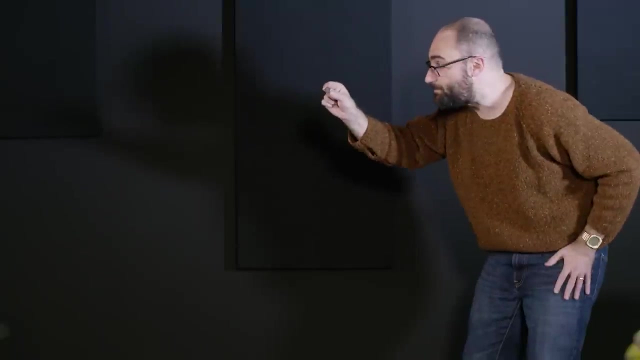 Anti-gravity, But not really. It's actually a demonstration of lenses law. Veritasium has a fantastic video on the topic, and I see it coming up on Reddit quite frequently, so I had to do it myself. It's really fun. These are very powerful magnets and I'm going to drop them, so 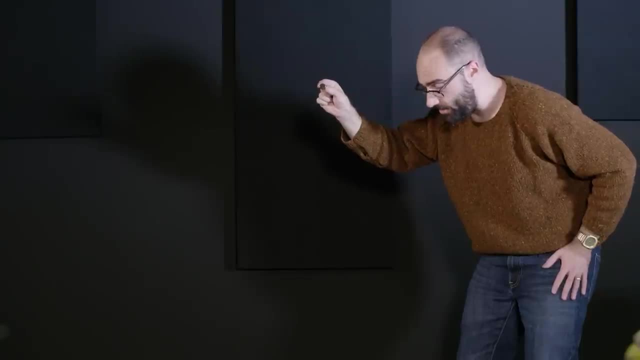 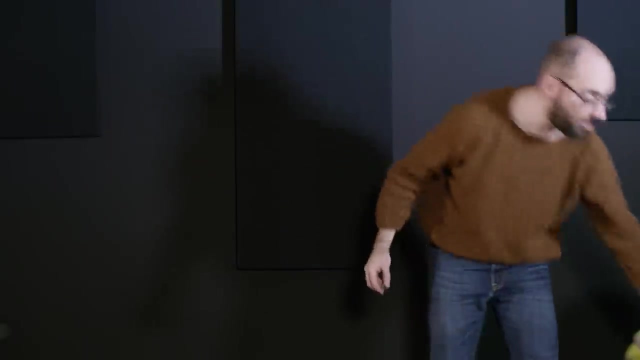 that they fall only due to gravity. Here we go: 3,, 2,, 1.. There it is: 9.8 meters per second, squared for those of you counting at home, But now I'm going to drop them through a copper pipe. 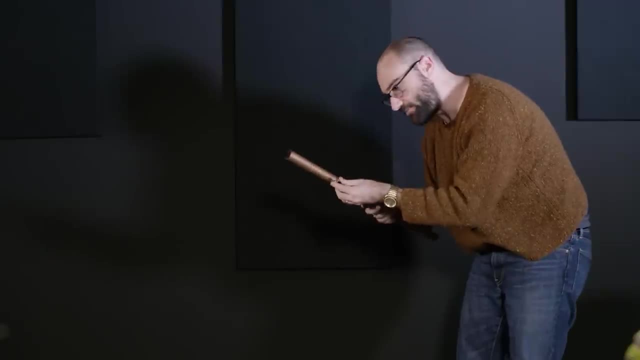 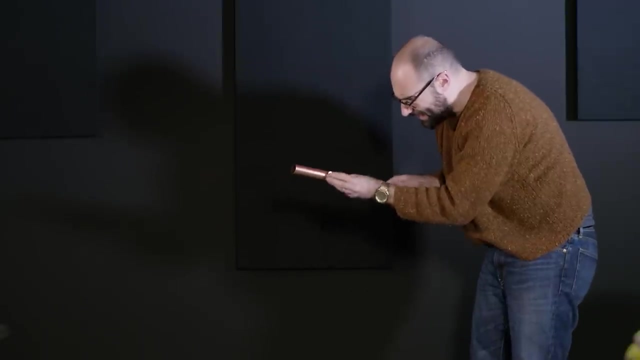 Copper has no interest in magnets. or maybe magnets don't care about them, Or do they? Well, we're going to find out. Notice that if I try to stick the magnets to the copper, it doesn't work, But if I drop them through, watch what happens. 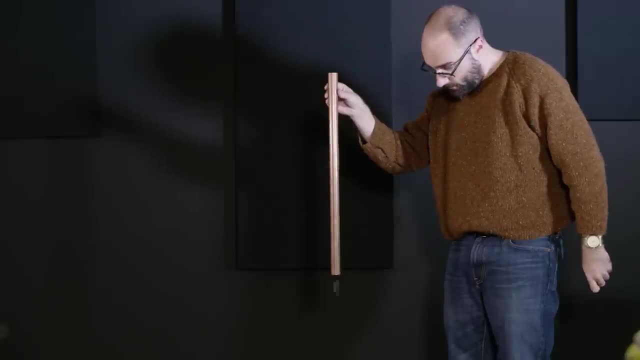 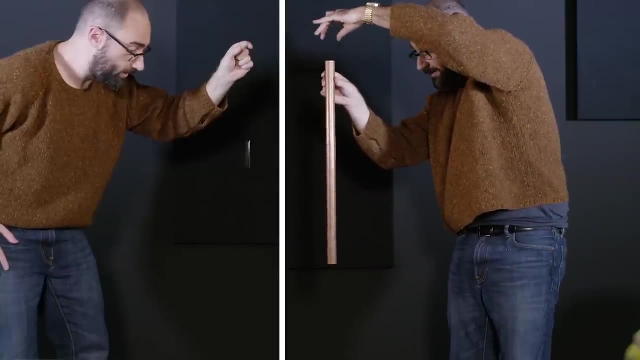 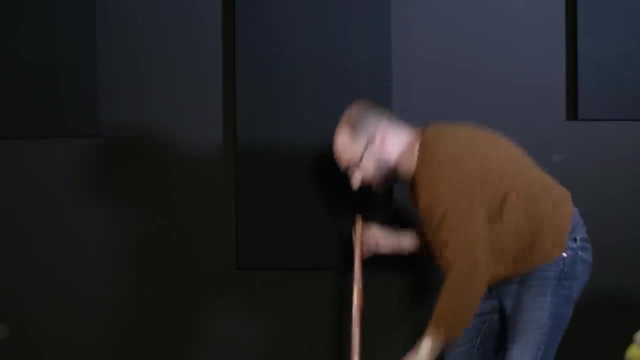 3,, 2, 1.. They fall really slowly. Here we go one more time: 3,, 2,, 1.. Something's slowing them down. You can hear that they are hitting the sides of the copper, but they don't have to do that. If my magnet was a better. 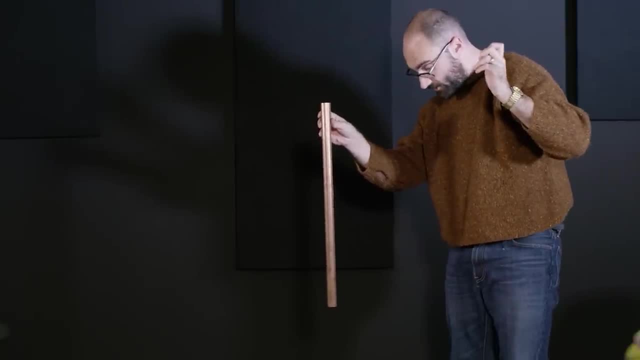 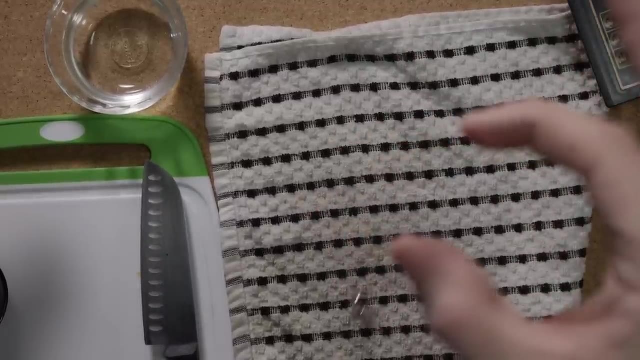 shape. it wouldn't happen And they would just glide right on down. They really are more slowly. Let's look at it from above. Here are the magnets being dropped by themselves. That's how long it takes for them to fall to the table. 3,, 2, 1.. 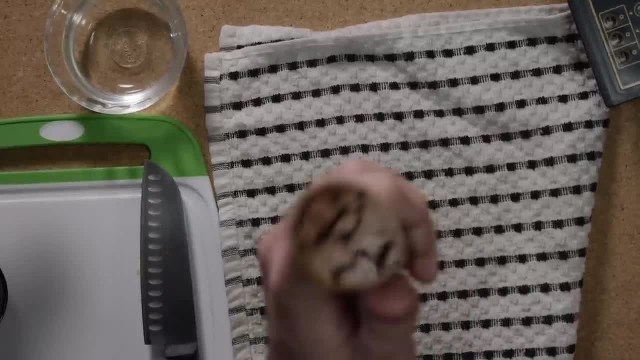 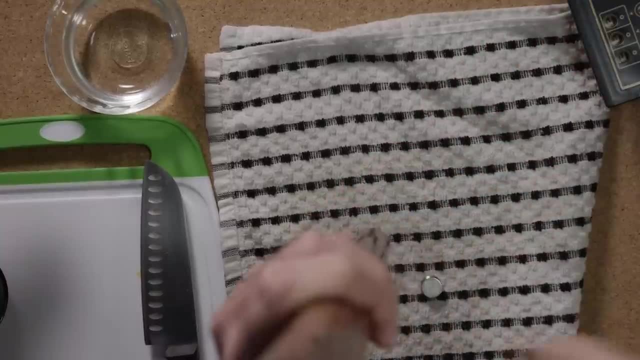 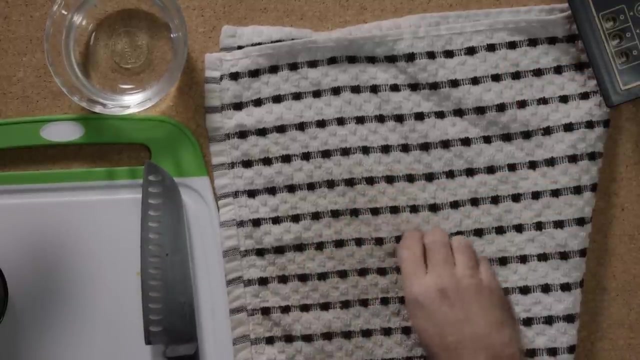 That's it. But now let's drop them through this copper pipe. Ok, ready, 3,, 2, 1.. Look at that. Let's try one more time: 3,, 2, 1.. two, one, And they hit Much, much slower. To see what's going on, let's play around. 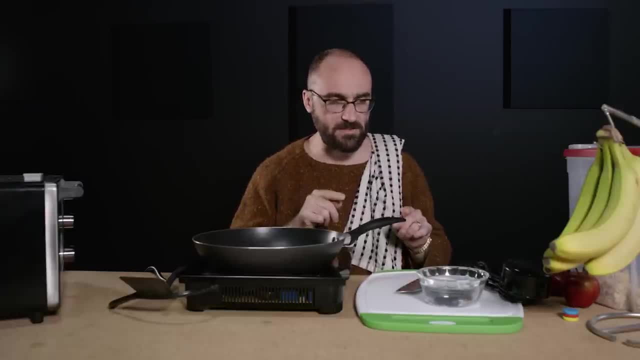 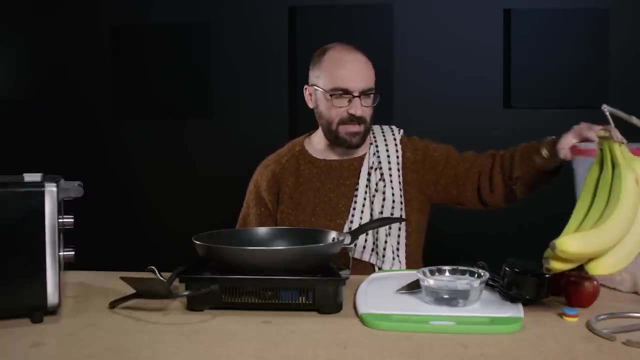 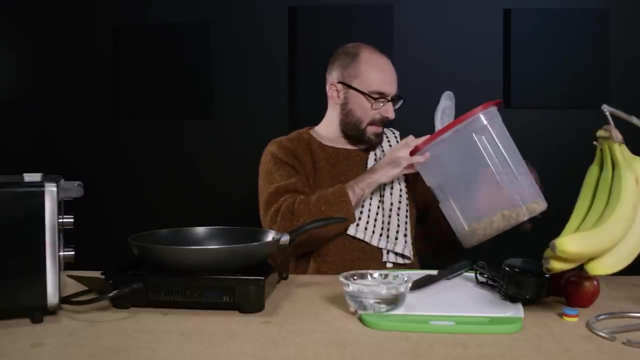 with magnets. One of my favorite magnetic fun recipes is one that I learned from Science Bob fantastic guy. It involves breakfast cereals and a bowl of water. So here's my bowl of water, And what I need to do is grab myself one little flake of this cornflake-like 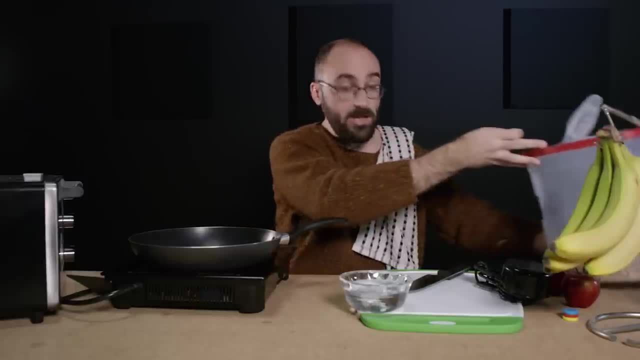 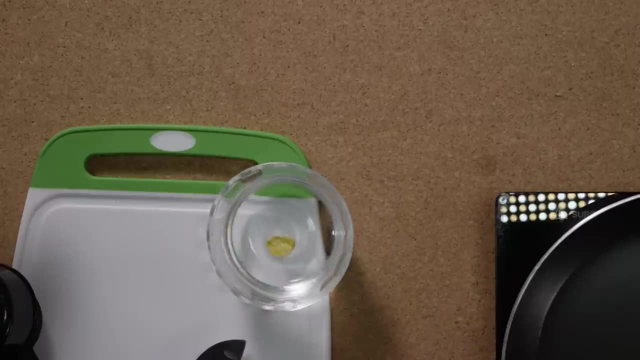 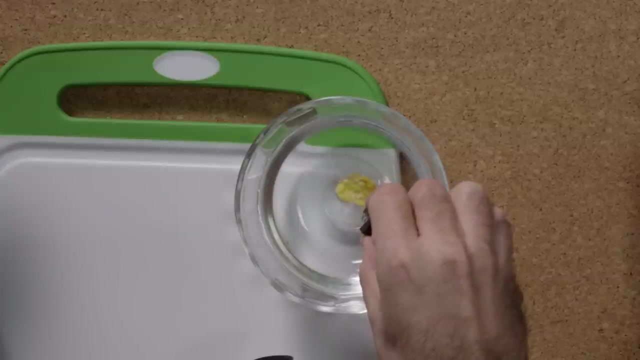 cereal. Now, many breakfast cereals are fortified with iron, And it's not iron in any kind of compound, It's literally just elemental iron. If I float a little piece of cereal there in the water looks pretty boring, But now let's bring a magnet near it. Oh look. 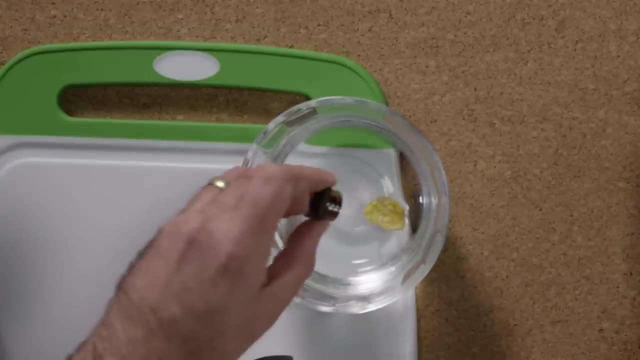 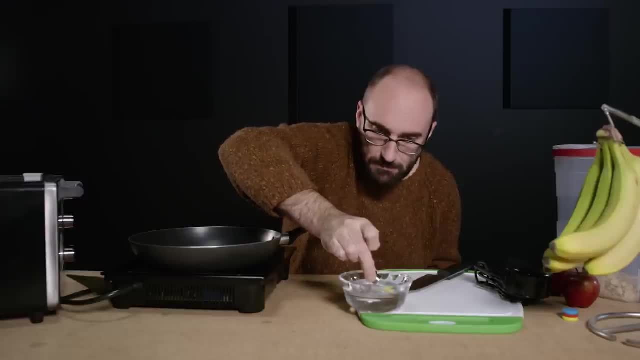 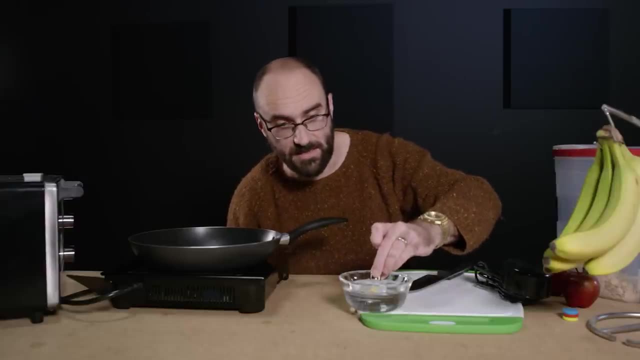 the iron inside it with a magnet. When you eat many foods, you're eating just straight up elemental iron like the kind we make nails out of, just like a lot less than would be in a nail. Oh, I love that. I hope it's clear for you guys to see. This demo wasn't really. 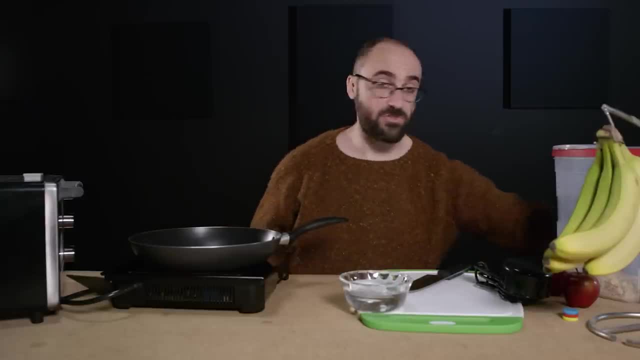 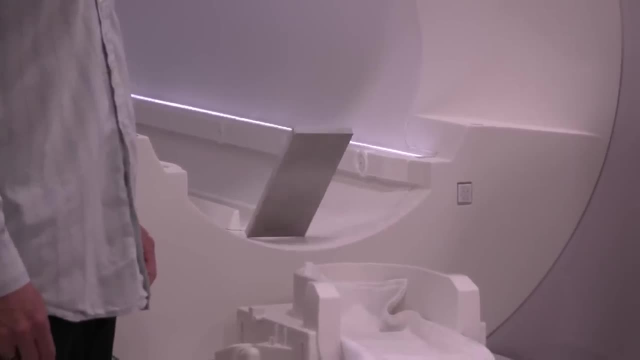 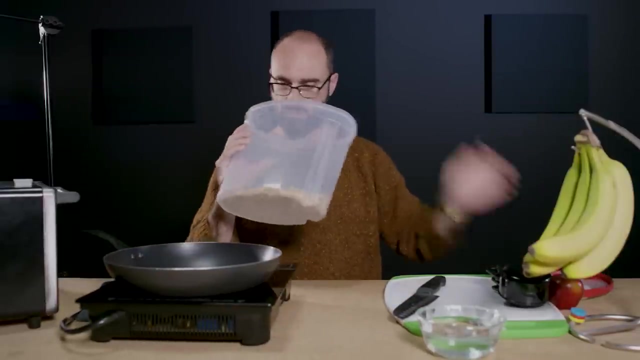 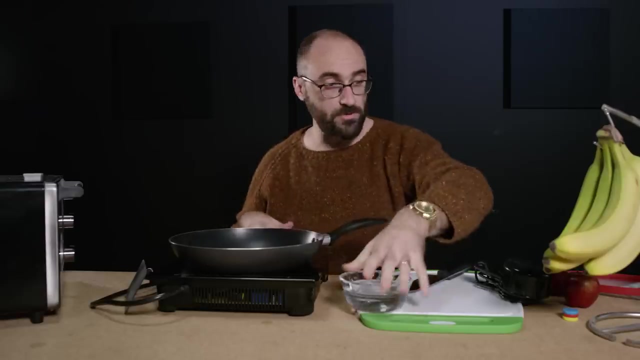 related to MRIs. I just thought it would be really fun to do To really start talking about why that block of aluminum fell so slowly around that strong magnetic field. we need a more advanced recipe, But I think you guys are ready for it. What we're going to need for this recipe is a really nice big nail. You're also 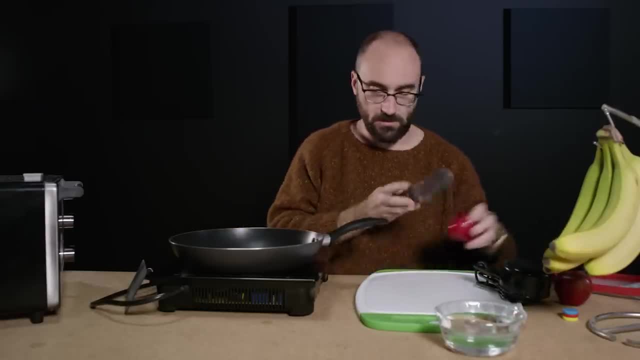 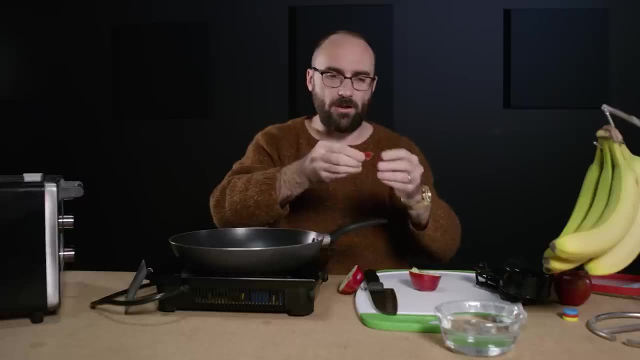 going to need. let's see this one looks good. Oh, perfect. Yeah, You're going to need some copper wire. It's thinly insulated. You might need more than this, but what you're going to want to do is take your wire. 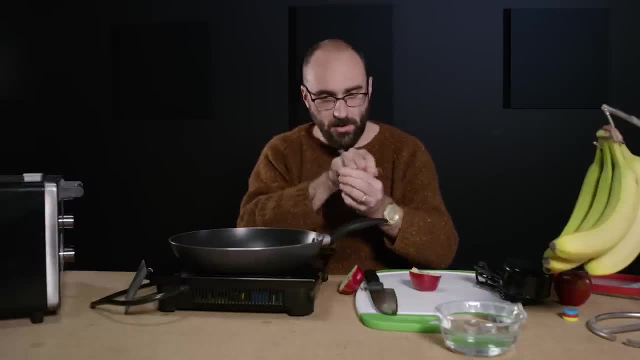 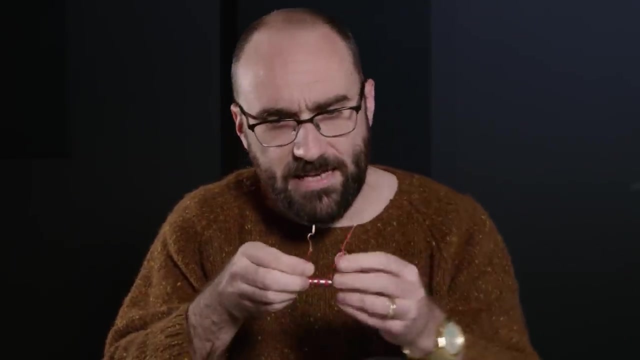 And coil it around your nail, Make the coil nice and tight, Keep them all bunched together so you can get as many wraparounds of the wire around the nail as you can get, And then, when you're done, you'll want to connect the two ends of the wire to a battery. Now that, 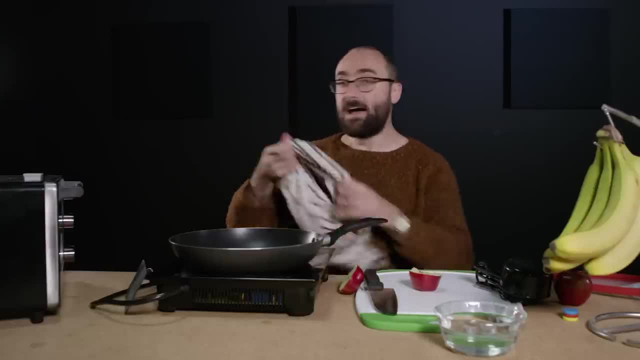 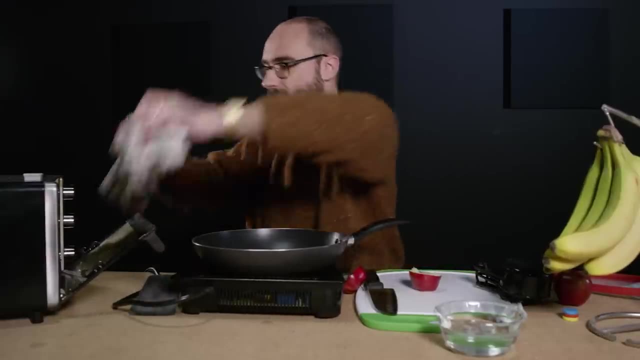 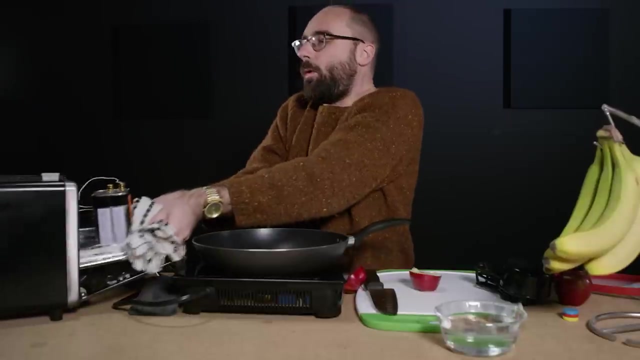 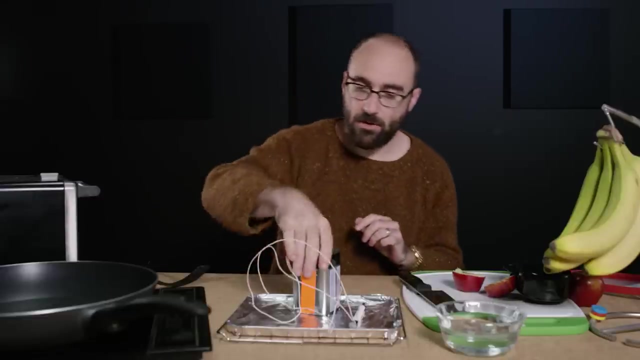 might take a while. So, because of the magic of a TV cooking show, I prepared an electromagnet earlier. Oh yeah, it's ready, This is good, This is really good, Perfect, Oh yeah, Hey, just like mom used to make, We've got here a big battery and 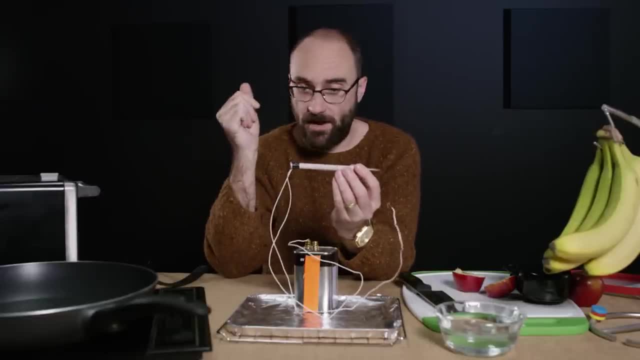 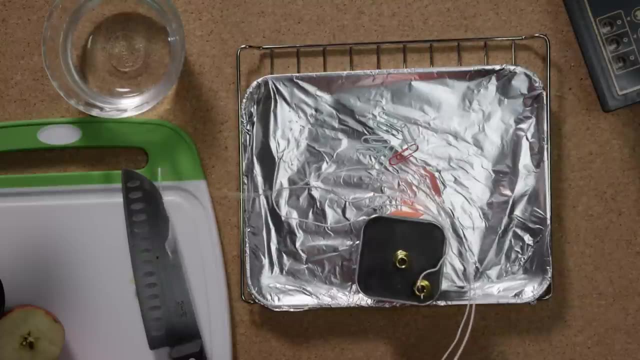 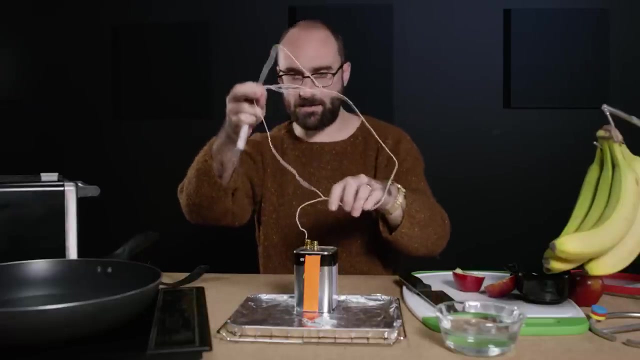 we've got a nail that is just coiled with lots and lots of wire. I think that we let the paper clips simmer long enough. I'm going to go ahead and put them there on our aluminum foil And I'll demonstrate that at this moment, because the wires are not completing a circuit. 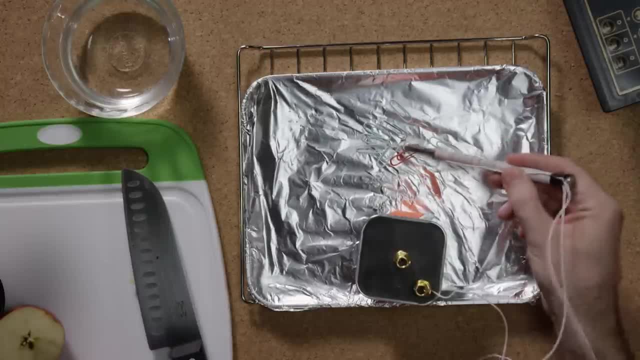 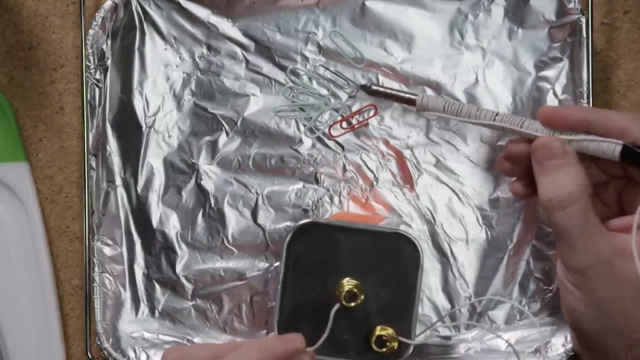 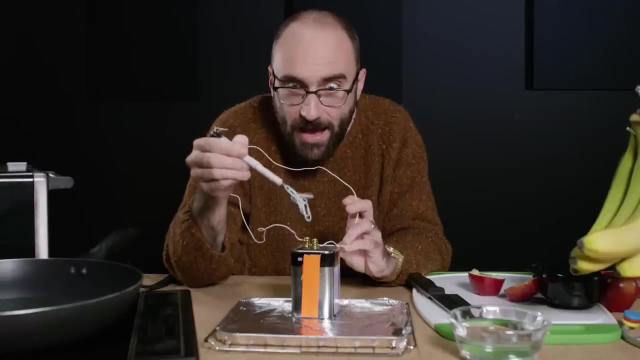 the nail is not magnetic. It has no effect on the paper clips, But now let's connect this wire to the negative terminal and see what happens. Okay, we're live, and yeah, Now let's turn off the current. Ooh, All right. 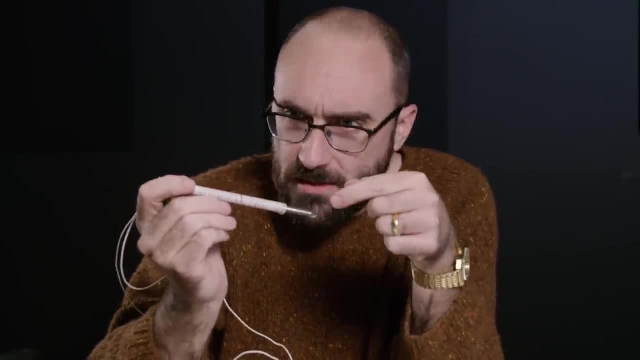 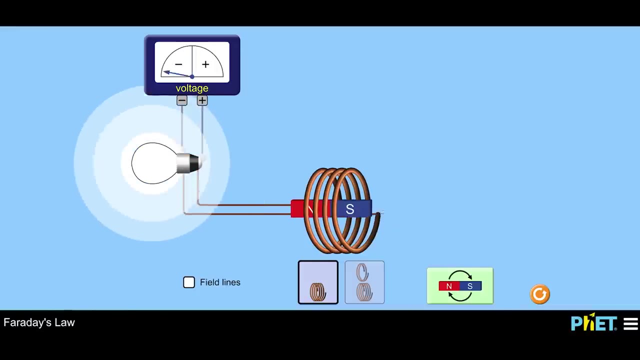 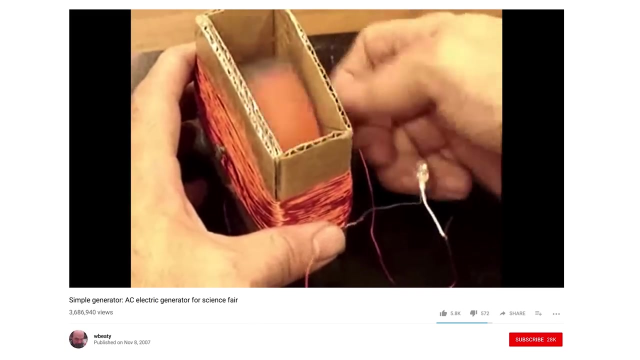 So what we've learned is that current flowing creates a magnetic field. What's even more fascinating is that a moving magnetic field can also generate electric current. There are fantastic videos online showing you how to do this. By simply spinning a magnet around a coil of wire, you can light a light up. This is how electric generators work All. 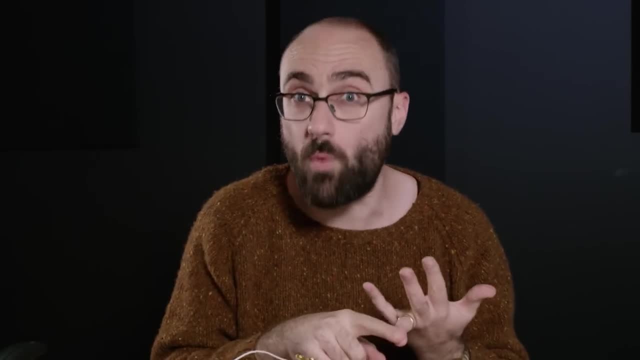 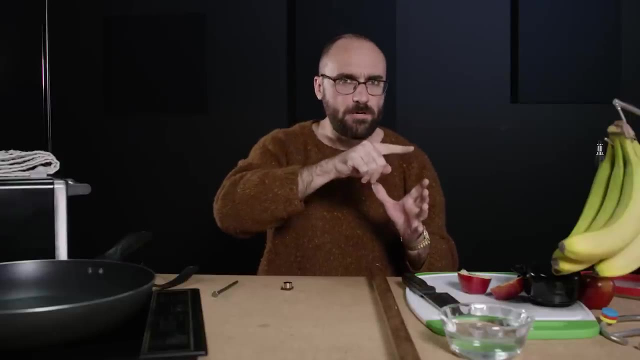 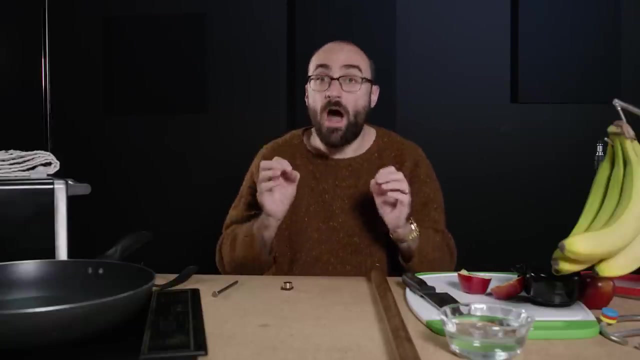 you need is something to keep the magnet spinning like wind or falling water, and your coil will supply electric current. There's a very interesting loop going on here. Electric current produces a magnetic field, but a moving magnetic field can produce electric current. Now THIS is KEY to WHY. 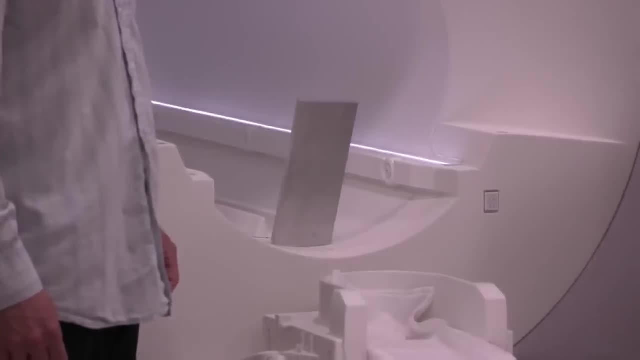 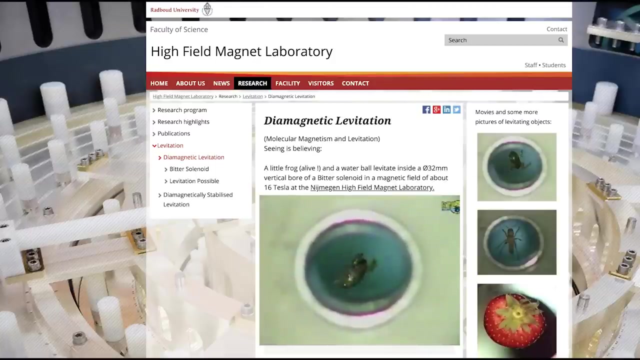 the block of aluminum falls so slowly near a strong magnet. It's also why even things like living frogs can be levated if your magnet is strong enough. Not all materials are attracted to magnets. This nail is made of iron and the magnet loves. 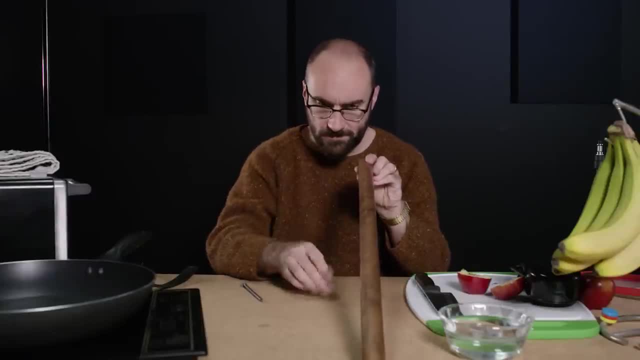 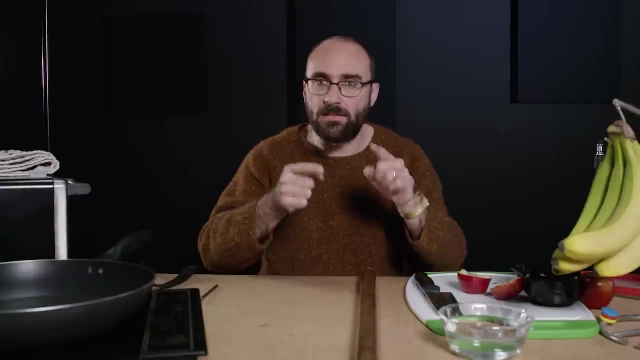 it a whole lot, Okay…, But this copper tube cannot do much. Never przywel tube nothing. the magnet just doesn't care at all. but what copper can do is conduct electricity. and since a moving magnetic field can induce electric current in a conductor, if we put these together and move one of them, well then. 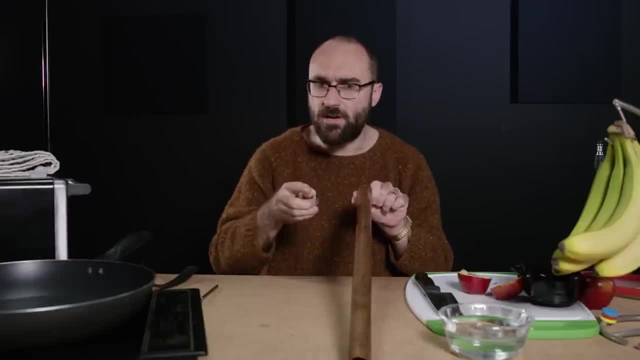 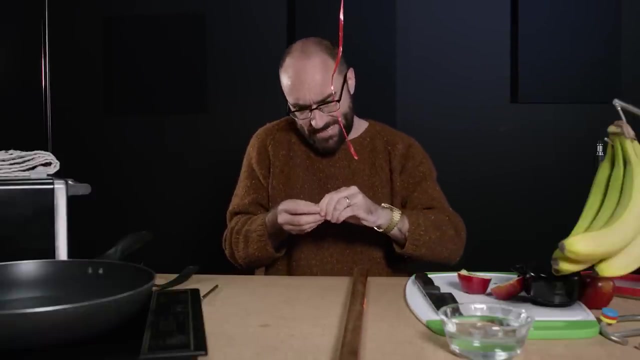 we should be able to produce some current, but we also know that electric current creates a magnetic field, which means we could make the copper act like a magnet by inducing current in it. let's try that using this conveniently positioned ribbon. I'm gonna take these neodymium disk magnets and very 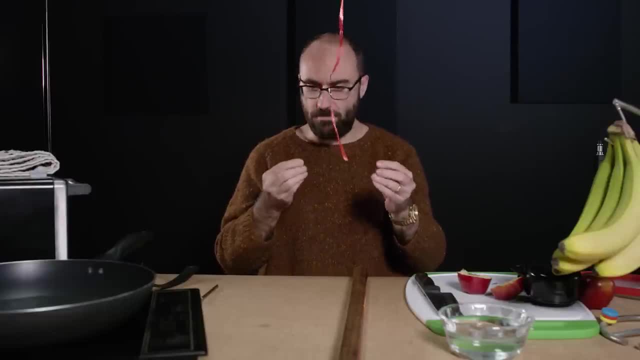 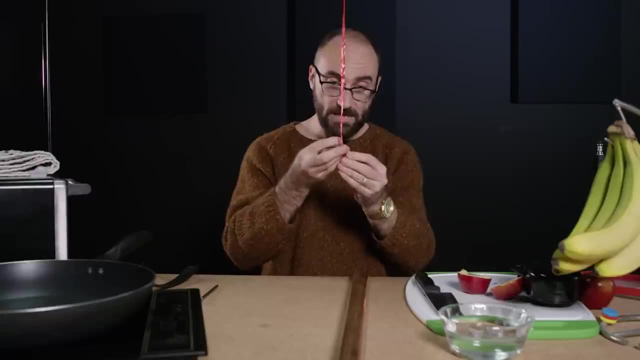 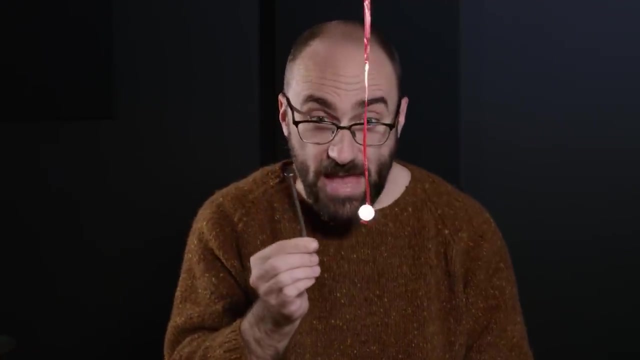 carefully slide them apart. it's very important to be safe with magnets. they they are attracted to each other so much more strongly the closer they get that they can easily pinch you. so please be careful with strong, mad magnets. okay, there we go. perfect, if I bring this nail near the 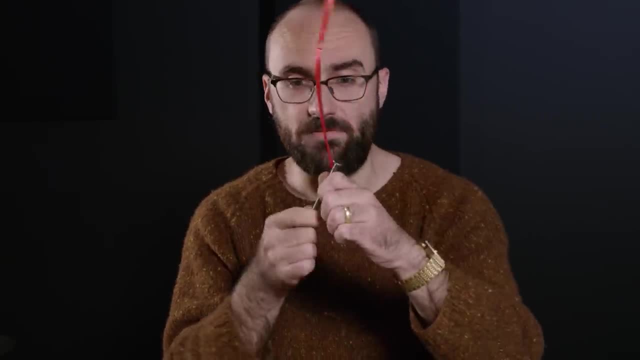 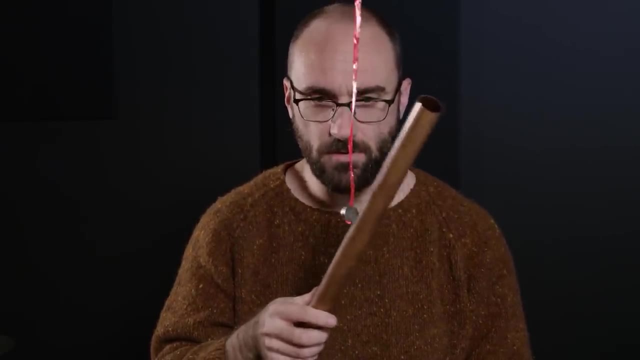 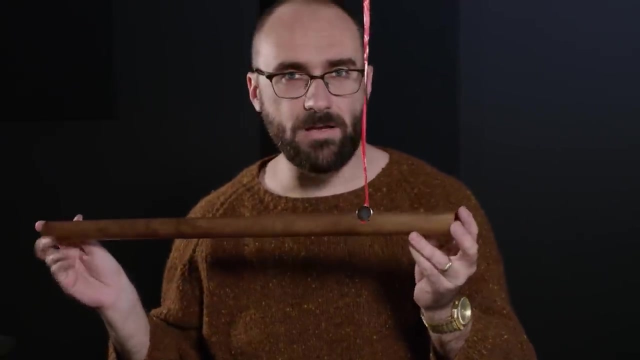 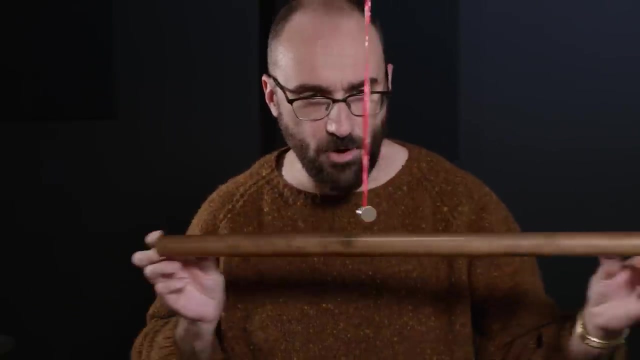 hanging magnets, who they love it, they love it. but the copper they don't really care much for, not not much interest. hello, wake up. no, they don't care. but watch what happens if I move this copper pipe quickly near the magnets. whoo, look at that. now they're not touching at all, but I'm able to get the. 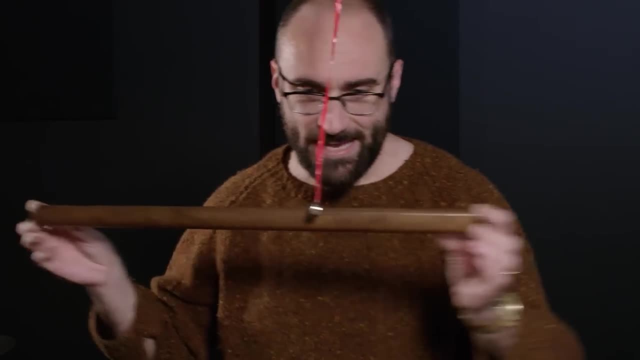 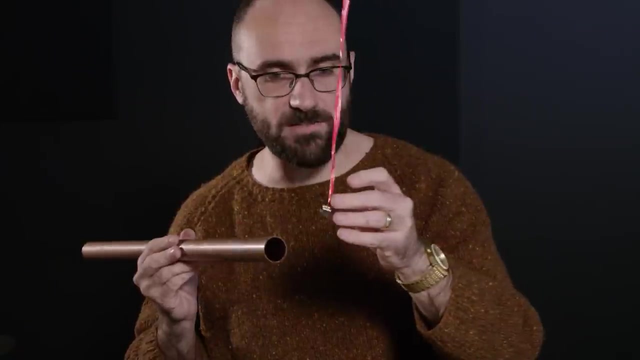 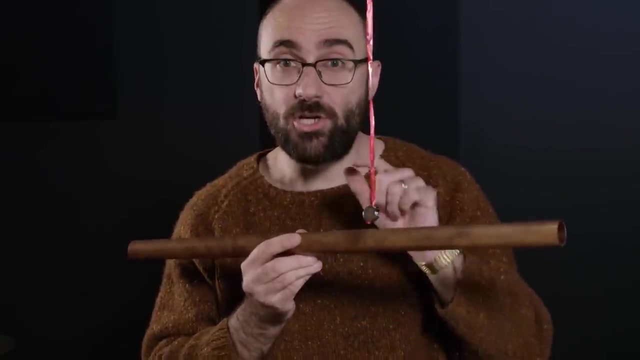 magnets moving, because as I moved the pipe across the magnets- look at that. well, it's really fun. as i move the pipe across the magnets, the magnetic flux density at each point along this piece of copper changes. that creates an electric current and that electric current by lindslaw will produce a 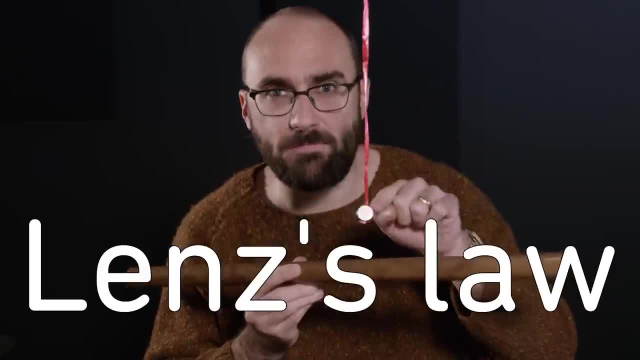 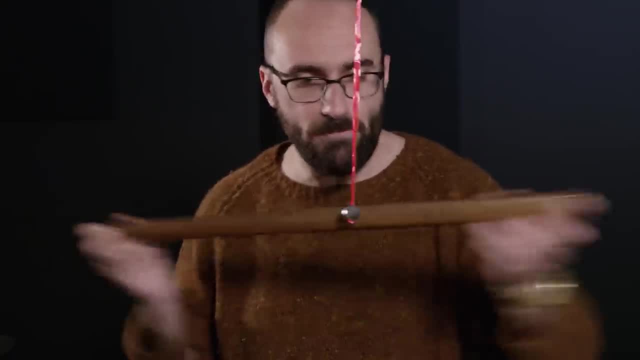 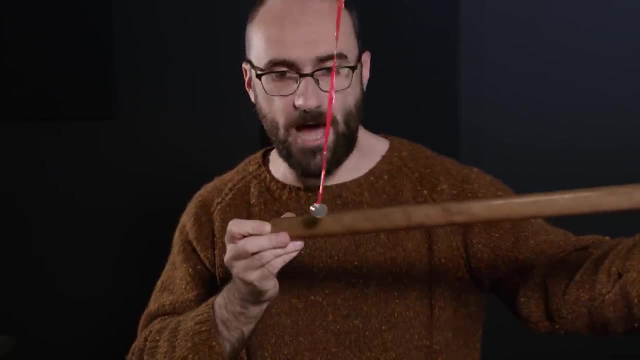 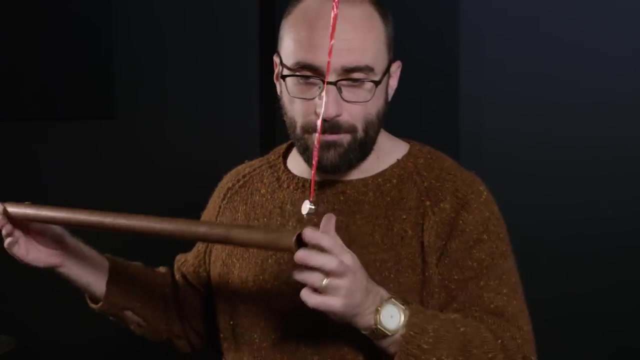 magnetic field that is opposed to the magnetic field of these magnets, causing hanging magnets to move. and the faster you move the materials, the more dramatic the effect. Oh yeah, beautiful. This is why the magnets fall through this copper tube so slowly. By Linz's law, the magnetic field they induce in the copper pipe is counter to their own. 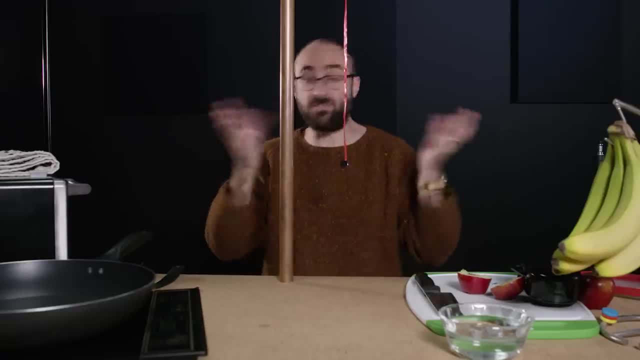 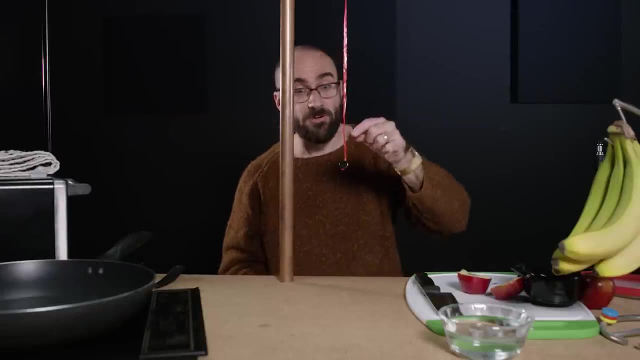 magnetic fields. You can think about this phenomenon in terms of conservation of energy. Where does the energy come from that produces the electric current in the pipe and the magnetic field? Well, it comes from the falling magnets. They fall more slowly because some of that energy is being converted into electric current. 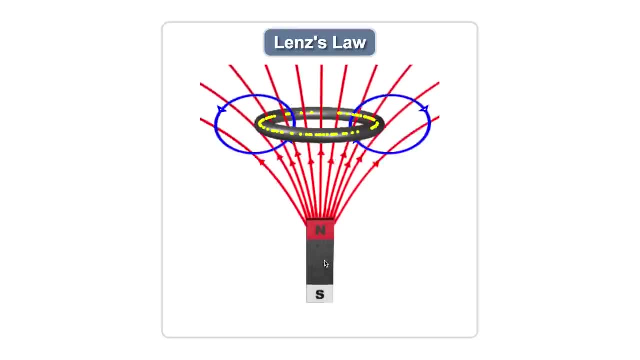 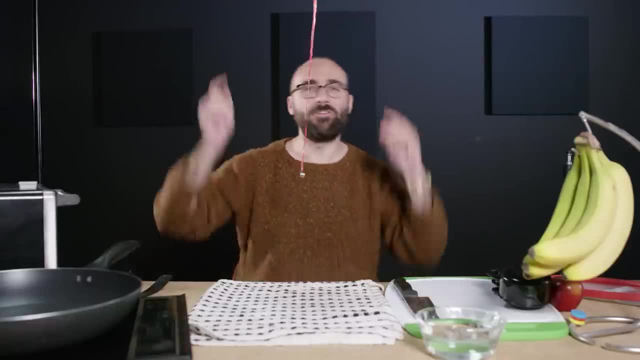 The currents created by a moving magnetic field are called eddy currents, And if you want to become more eddy-cated about them, there are links down below where you can learn more. Now let me address a quick question you might be having. 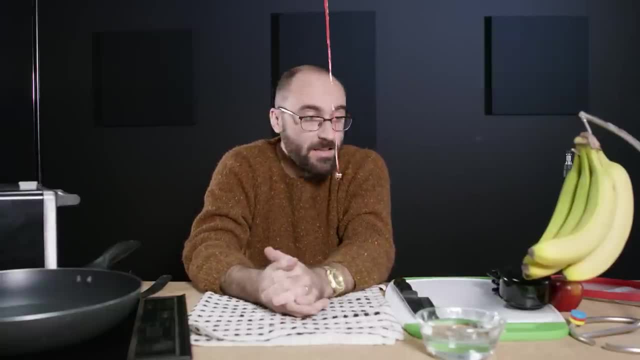 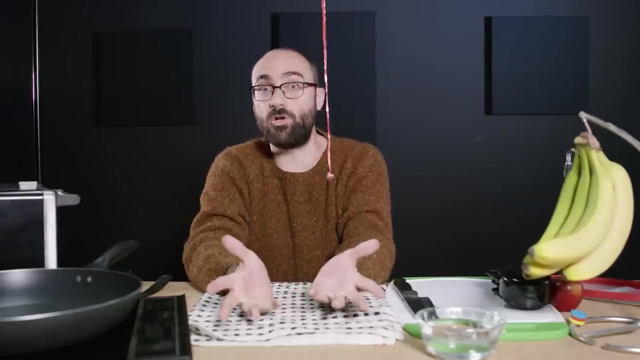 Why is a video like this on the DONG channel and not on Vsauce1?? Well, I answered this question on Reddit yesterday And the long and the short of it is that in my opinion, both channels have sort of the different goals. 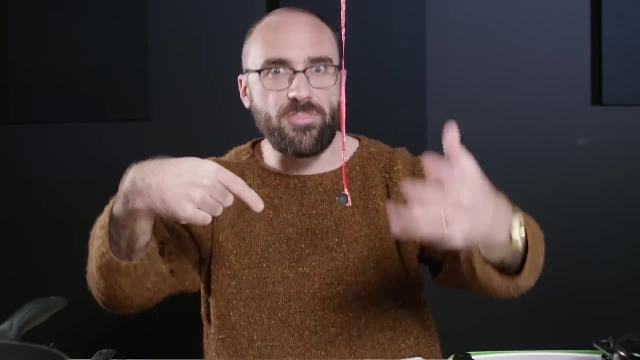 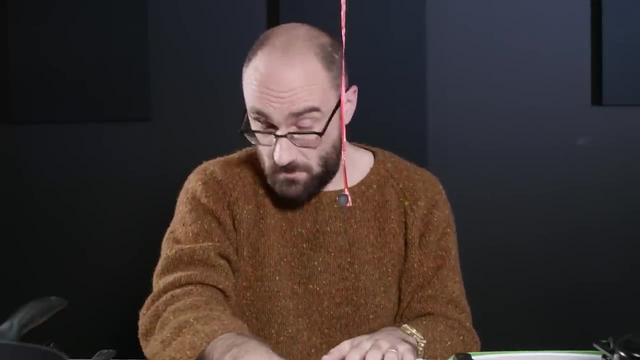 My goal on Vsauce1 is to upload videos where I get to share the things and the new framings that caused a concept to finally click in my head, Concepts that I never thought I'd be able to wrap my head around before. Now, doing that can take a long time. 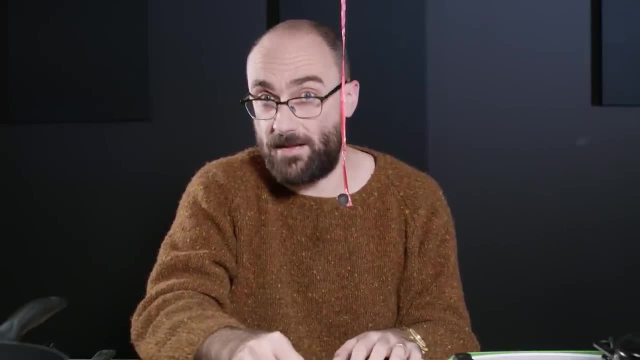 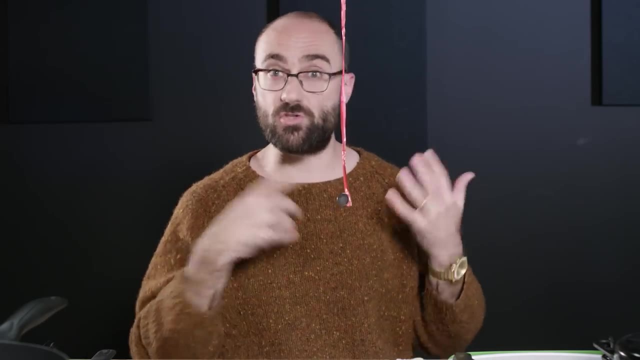 I've been working for a while on an episode about rotational phenomenon, specifically some counterintuitive ones, And I'm not happy on Vsauce1 just using vocab words like torque and moment of inertia to describe what's going on. I want to define what those words mean. 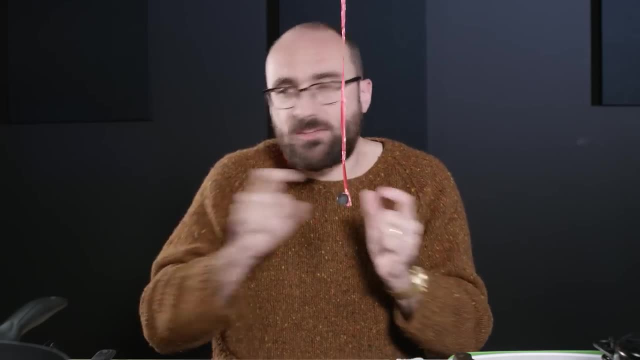 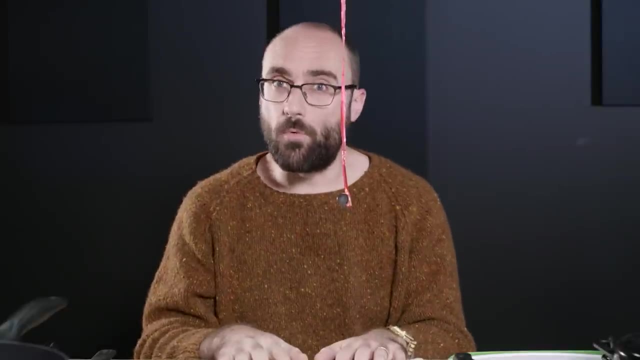 And ask why, over and over again, so far back that we're left with nothing but geometric principles and symmetries of the universe. That can take a while. So thank you for your patience. I hope that you share my passion for the topic when the episode comes out and think that 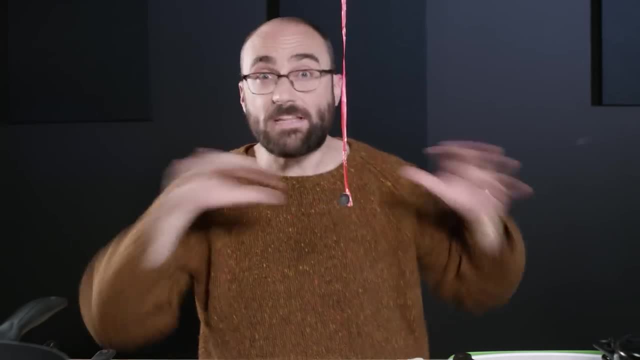 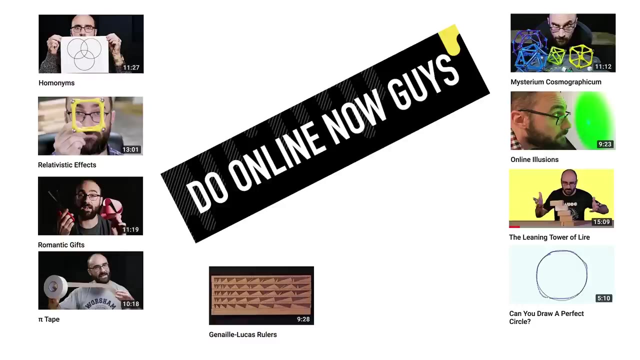 it's worth it, But on the DONG channel I'm able to share things really quickly without disappointing people who expect something deeper. In fact, in this year so far- in just 2018, I've already made now 10 episodes on DONG. 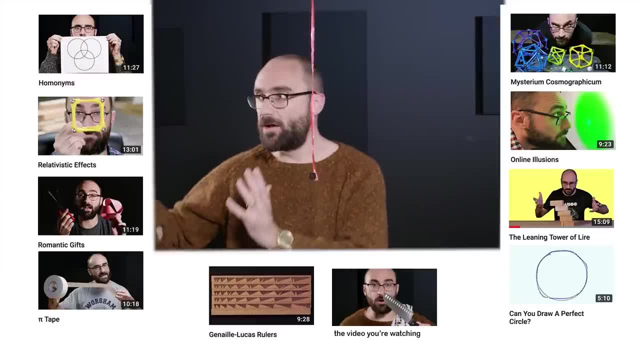 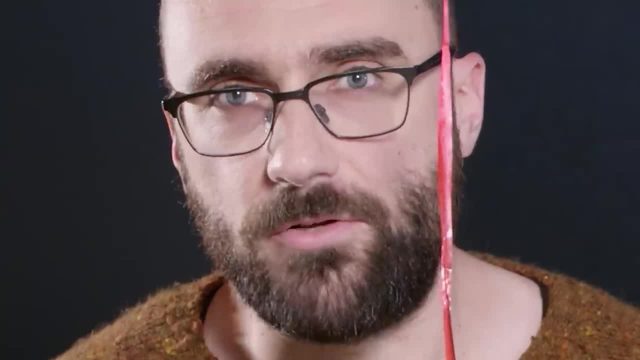 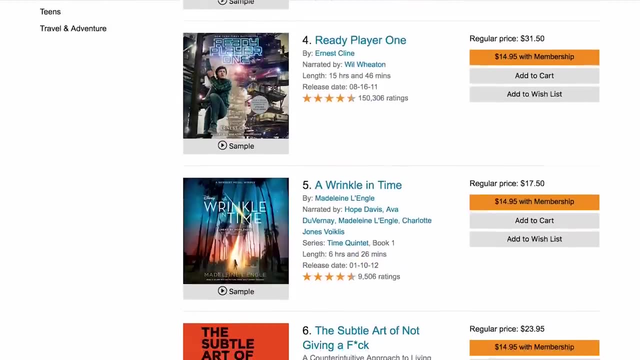 That's more than I made on Vsauce1 all of last year. So I love DONG, But I remain steadfastly committed to both channels. Now DONG is made possible, especially today, by our sponsor, Audible. Audible contains, I mean, just an unmatched collection of audiobooks. 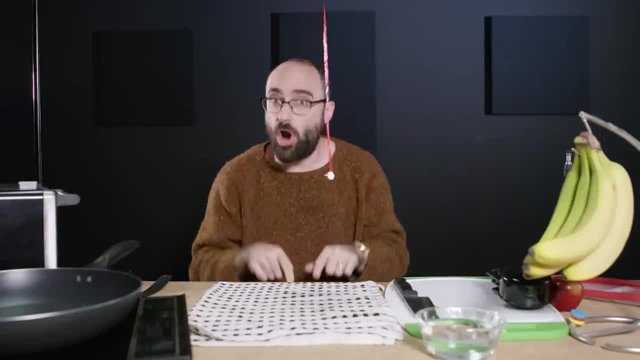 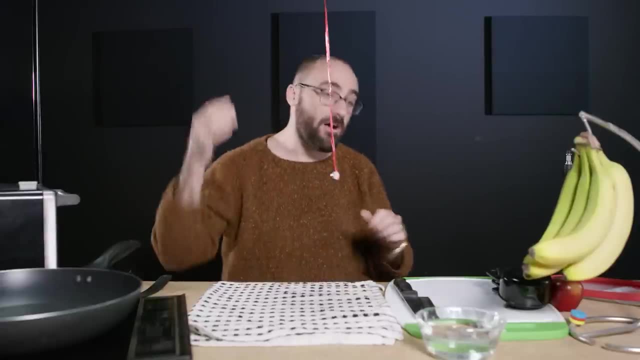 As you guys know, I love reading And now that I live in LA I'm in a car a lot, So audiobooks come in extremely handy. Audible is offering you guys out there watching Michael's Toys today A free audiobook. 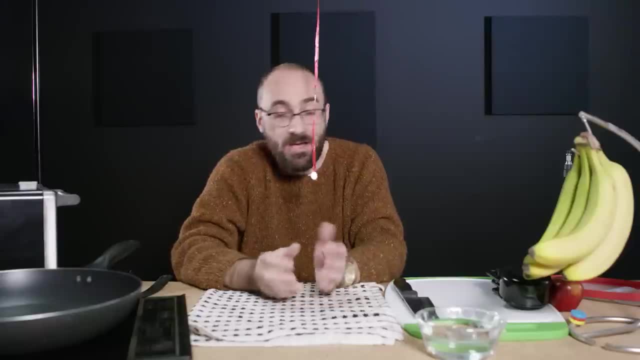 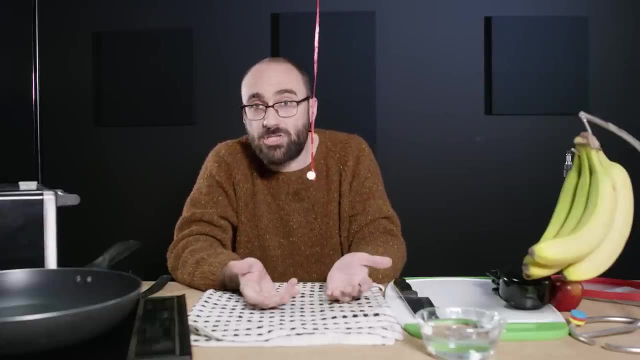 A free audiobook download with a 30-day trial membership. What's great about Audible is that when you download an audiobook, it's yours to keep forever. Okay, If you end your membership, you still own the book. It's fantastic. 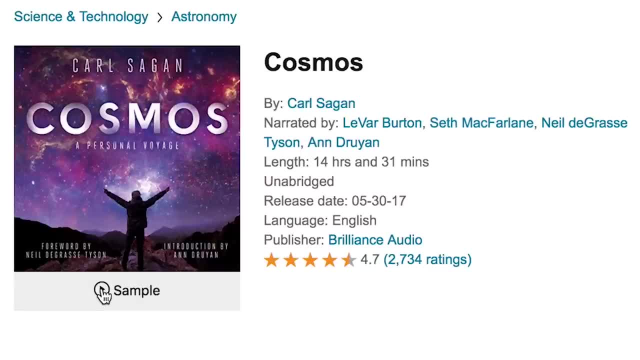 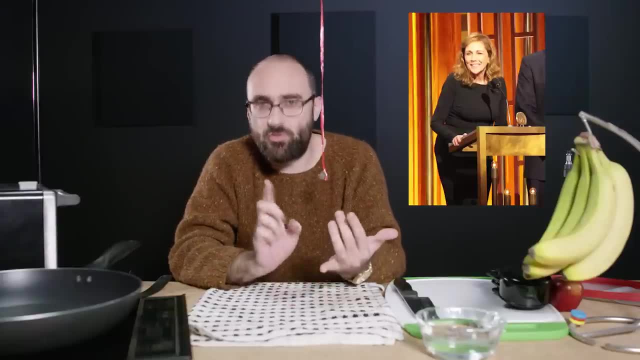 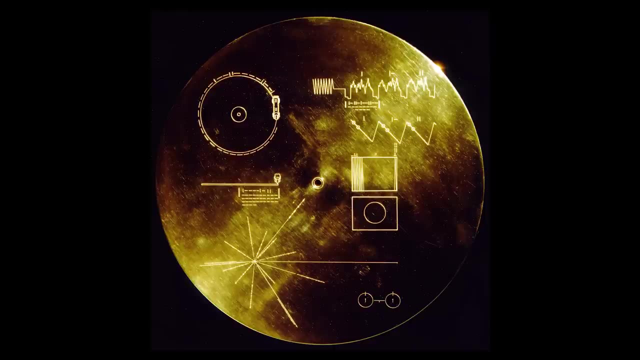 I would highly recommend the audiobook of Carl Sagan's Cosmos. The voices narrating it are just unbeatable. One of the narrators is Ann Drian. She was the creative director of NASA's Golden Records project that put the Golden Records on Voyager 1 and 2.. 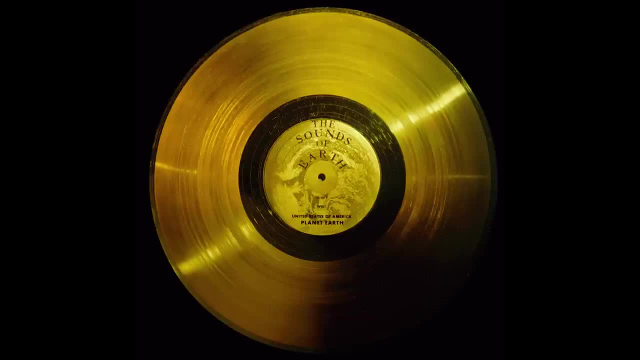 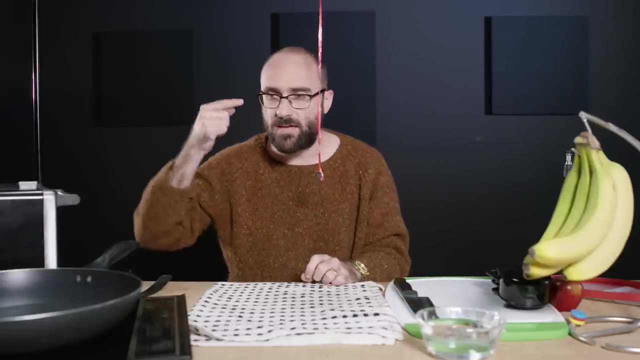 A recording of her brainwaves are on that record that someday other lifeforms out there might find. While she had her brainwaves recorded, she was thinking about the history of Earth civilizations. She was thinking about the problems that we face here on Earth. 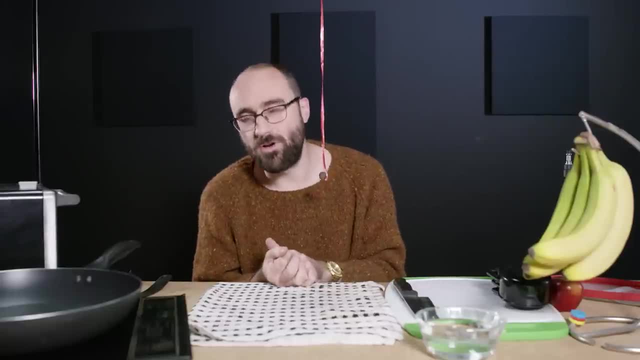 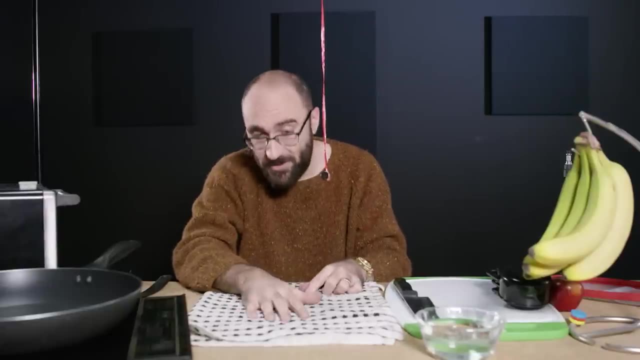 And she even thought about what it feels like to fall in love. Wonderful stuff. She co-wrote Cosmos, the documentary, and a year later married Carl Sagan. But it's not just her voice on there, It's also got Neil deGrasse, Tyson LeVar Burton, Seth MacFarlane. 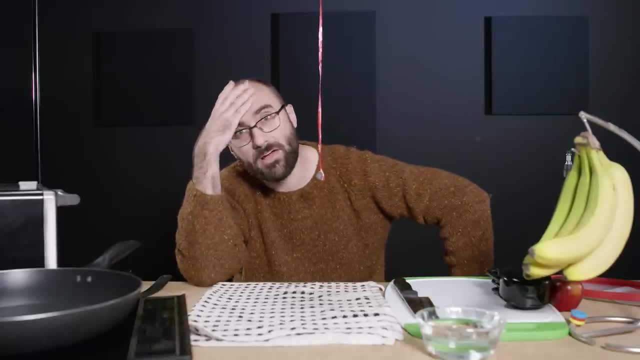 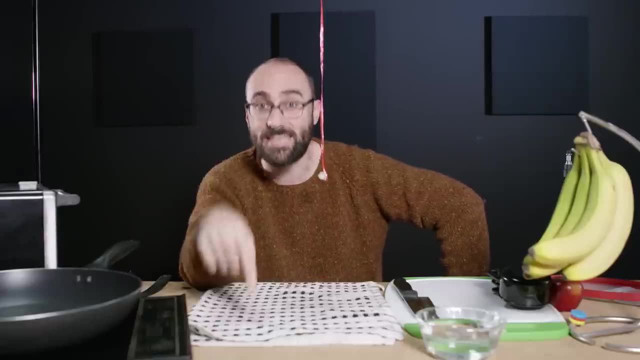 It's amazing, I mean holy cow. I totally hugely recommend that By going to audiblecom, slash Michael's Toys, you can take advantage of the offer we have today. You can also text Michael's Toys to 500-500.. Awesome stuff. 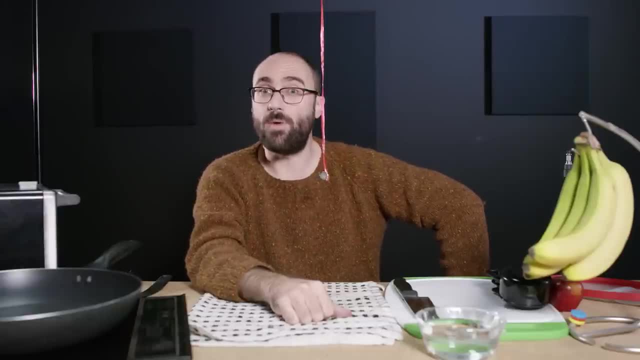 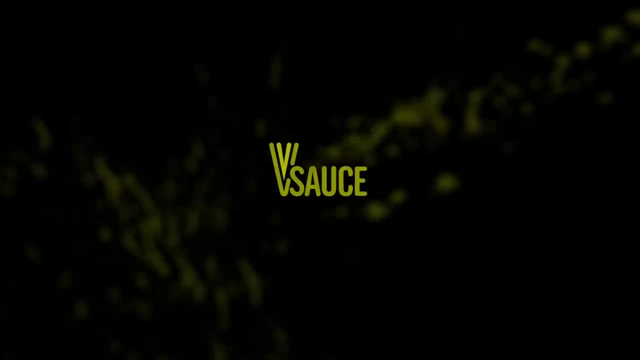 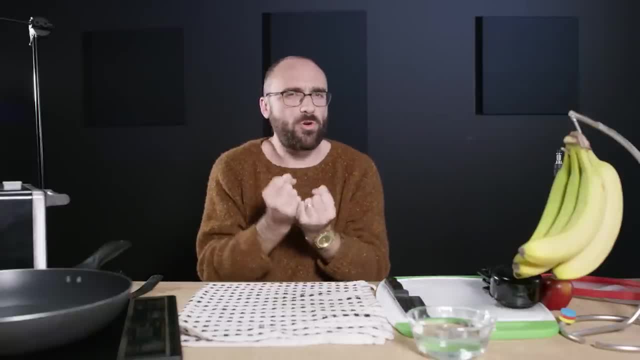 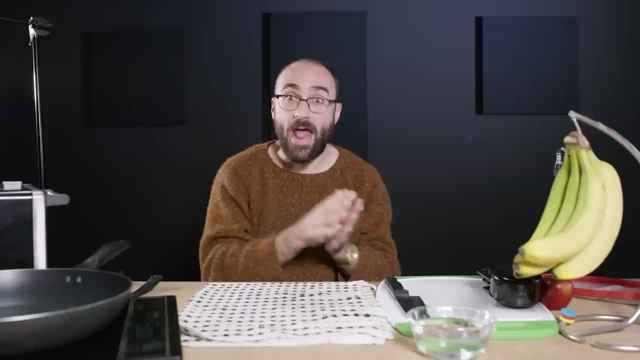 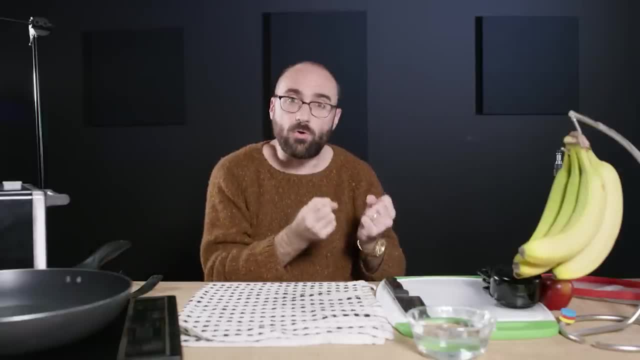 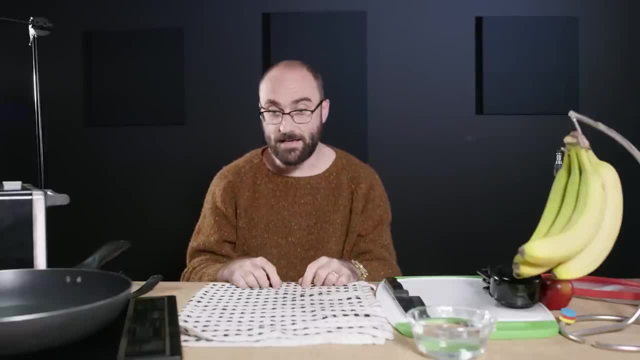 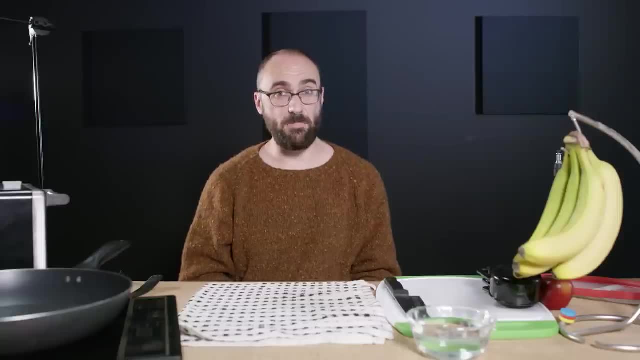 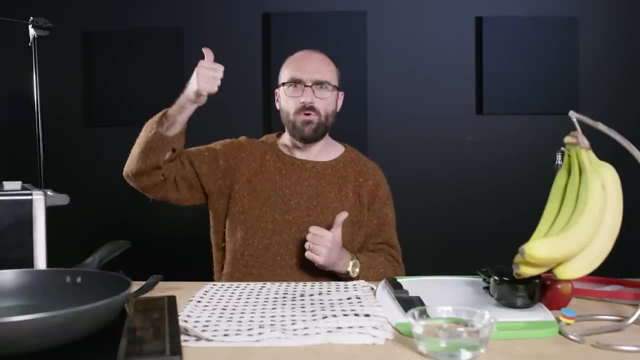 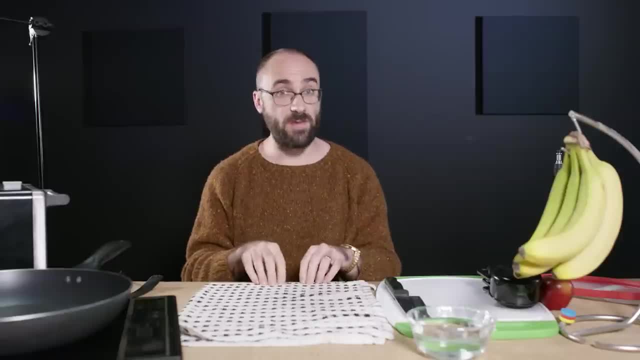